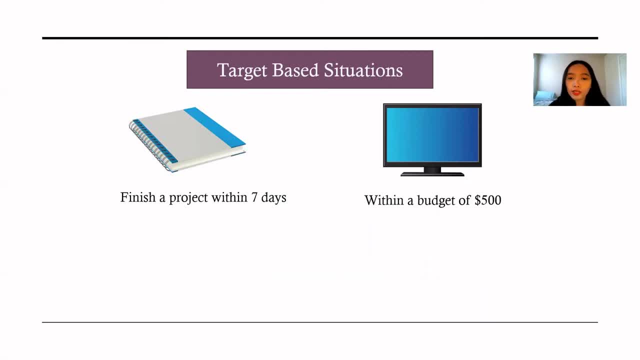 either be finishing a project within a week or trying to buy a TV with a pre-decided budget of $500.. So the question now becomes: what is the objective for both situations? Well, for the first situation, the objective is to try and get as much points as possible on the 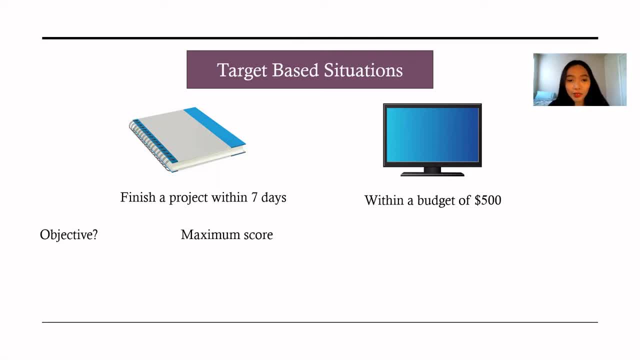 project For buying the TV with a minimum budget, the objective is most likely to minimize the cost. So what are our constraints or what are we limited to in terms of our choices for both situations? Well, for the first one, we are limited with time. 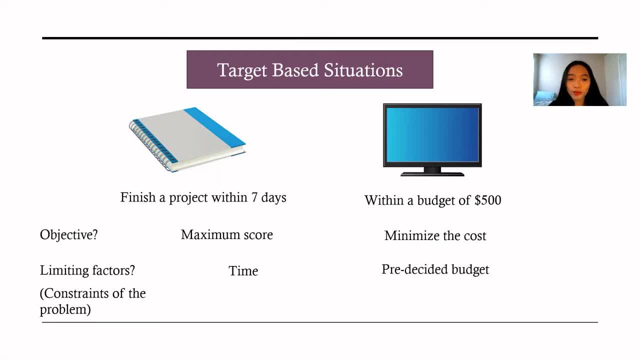 While the second situation- we are limited to a budget that we have decided initially. So for problems like this, where we have an objective which is either to maximize or minimize something under a certain set of constraints, we call these problems optimization problems. And the way we solve optimization problems is well, there are numerous ways, but 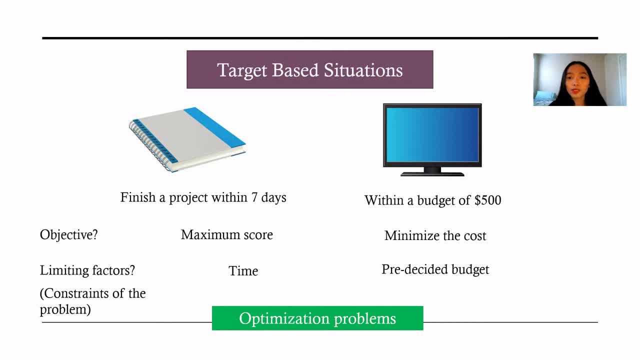 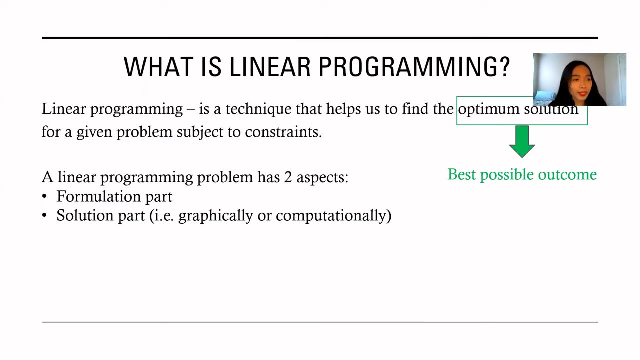 in general, we call the methods for solving optimization problems optimization problems, And one of the most famous optimization techniques available is linear programming. So linear programming is a technique that you use to solve optimization problems. It solves for what we call a global optimal solution, or the solution that provides us the 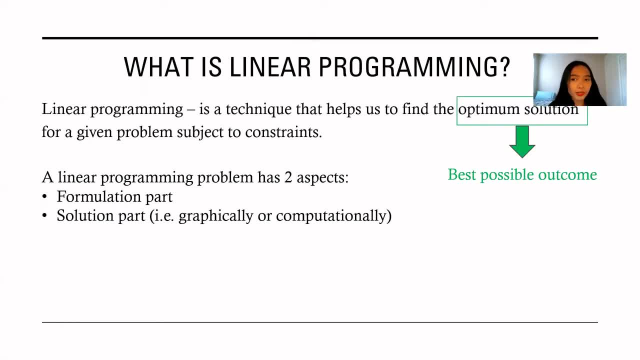 best possible outcome. So a linear programming problem usually has two major aspects. This is the formulation part, wherein we take in a real-life problem and convert that to a mathematical problem, And then we take in a real-life problem and convert that to a mathematical. 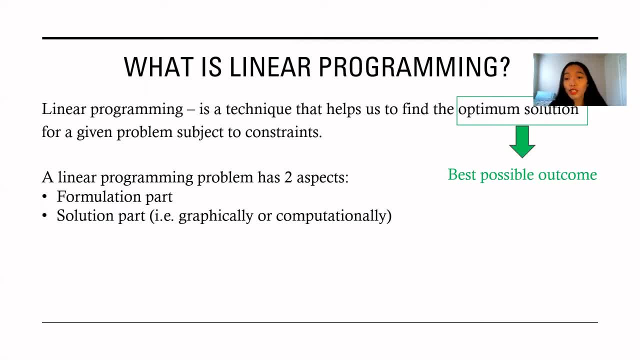 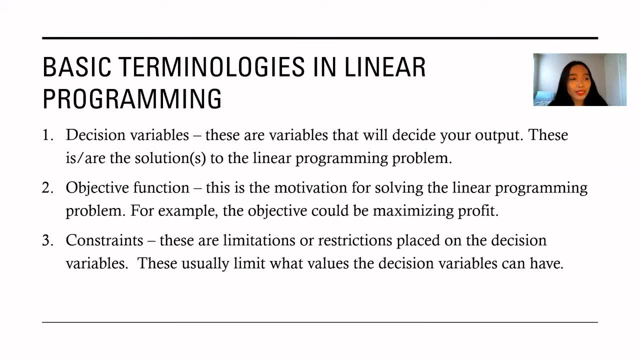 problem which we then solve either graphically or computationally. So basic terminologies we need to know about linear programming, So we have what is called a decision variable. Our decision variables are also known as our unknowns for the problems, And our unknown variables depend on what kind of outcome we want to obtain, And so our outcome. 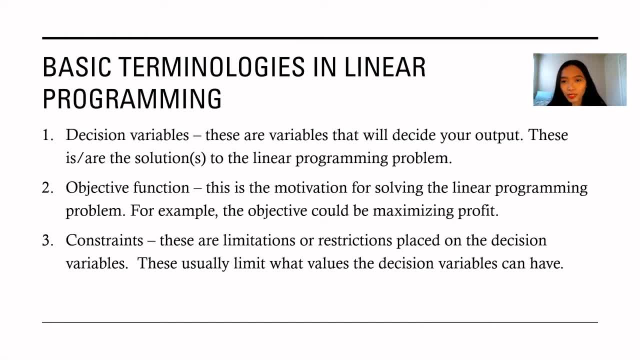 or our motivation for the problem is what we call the objective function, And so we want to decide aren't going to be the objective function of the problem, So we have to have the objective function, And there's also a developmental problem to solve it. So when we're developing an optimization problem, 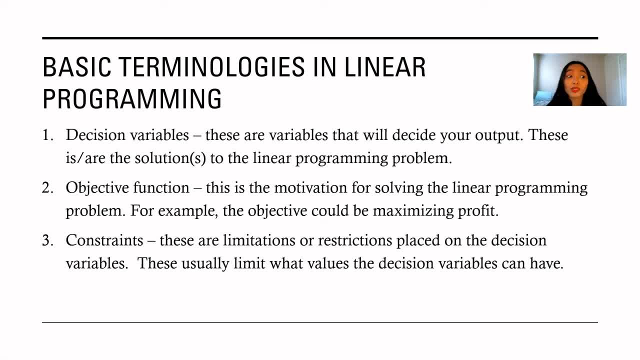 we have two basic coordinators and then we have two analytical combinations. We have the biographical decision variables, based on what our objective is, or what our objective function in this case is, And our decision variables. our choice of our decision variables is limited to constraints. 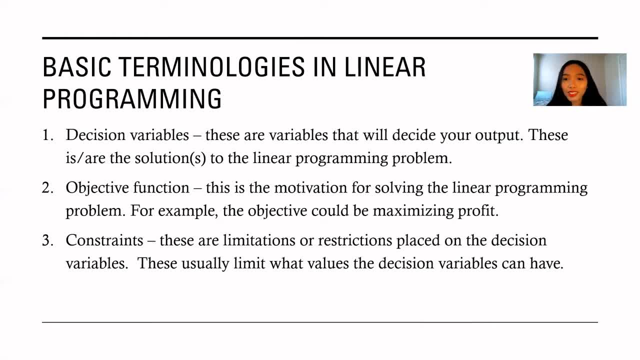 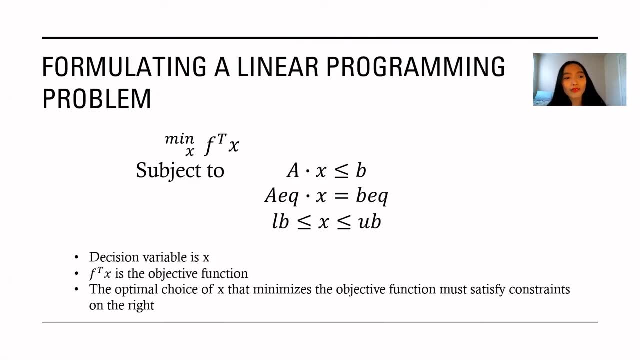 So our decision variable needs to be able to satisfy all these constraints and meet the objective function to be able to consider this solution to be the most optimal solution for the linear programming problem. And so when we formulate a linear programming problem, it tends to have this form, wherein our decision variable x is here and we want to find our 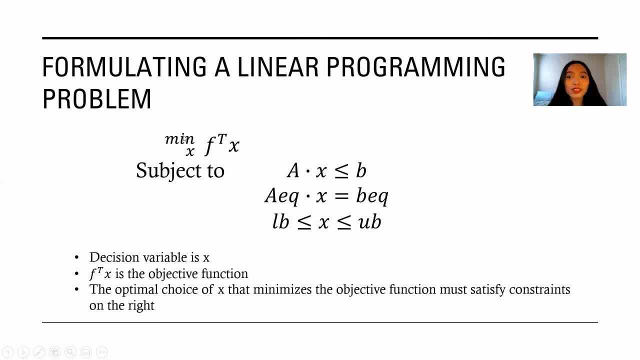 decision variable x that minimizes or, in some cases, maximizes our objective function denoted by f raised to t times x, given that this decision variable x satisfies numerous constraints. These constraints can come in the form of inequalities, equalities, and our decision variables tend to have a predefined range. 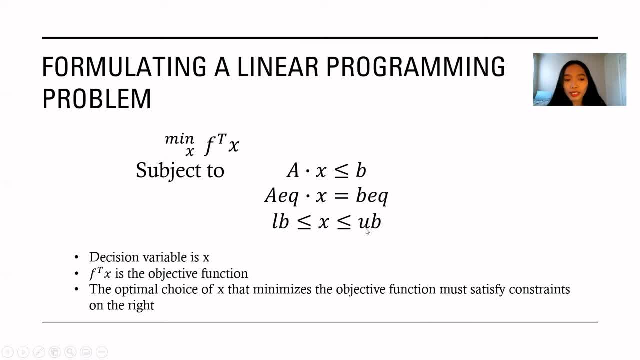 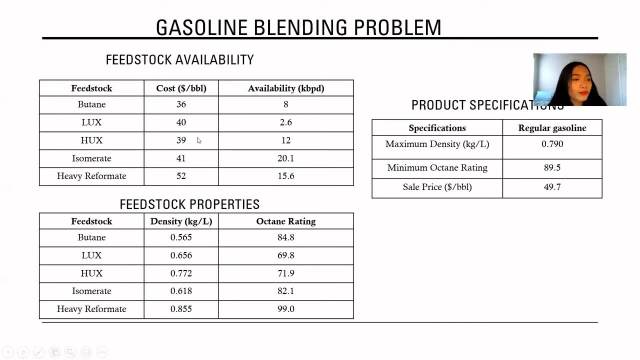 in terms of the options that it could be. And so let's look at a gasoline blending problem. So say we are given five feedstocks: butane, LUX, HUX, isomerate and heavy reformate. The problem asks us to determine the optimum amounts of each of these five feedstocks that we need to mix. 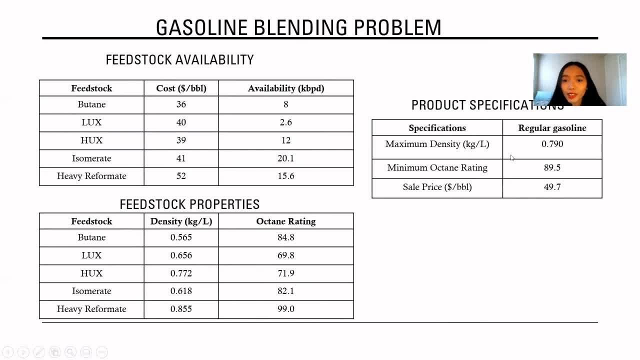 together in order to obtain a desired regular gasoline product that has the following specifications for its density and octane rating, and with the sale price of $49.7 per barrel. So, given this objective, we know what the cost of each of our five feedstocks are per barrel, and how much of them. 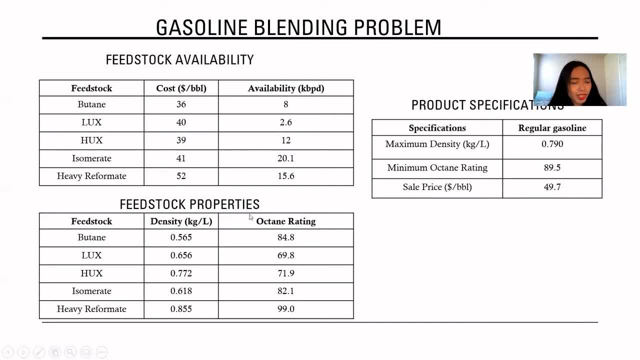 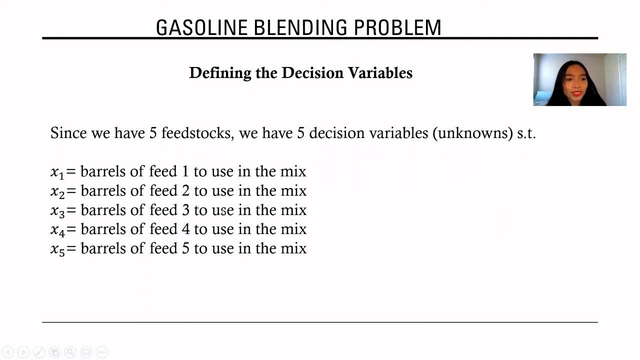 are available for use for mixing, And we are also given information about the densities and the octane rating for each of these five feedstocks. So what's our decision? variables, Well, our knowns, and this case are the amounts of the five feedstocks that we need to mix together to make the desired. 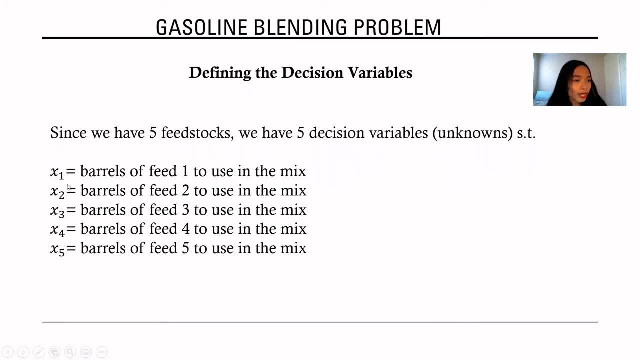 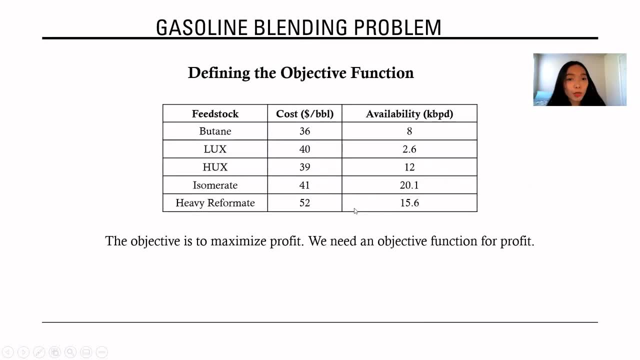 gasoline that provides the maximum profit. So X1 to X5 refers to the unknown amounts of barrels of each of our feed that we need to mix Objective function. So the objective function, or the objective rather, for this problem is we want to maximize the profit for this gasoline blending. 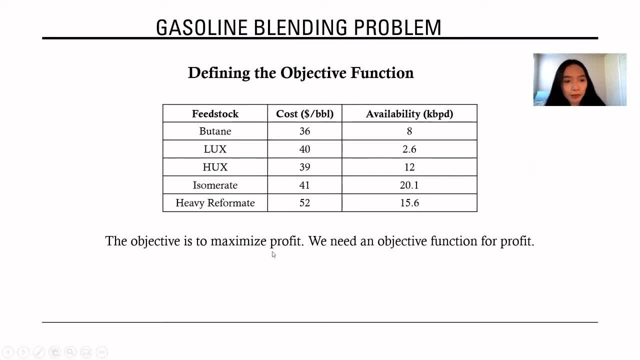 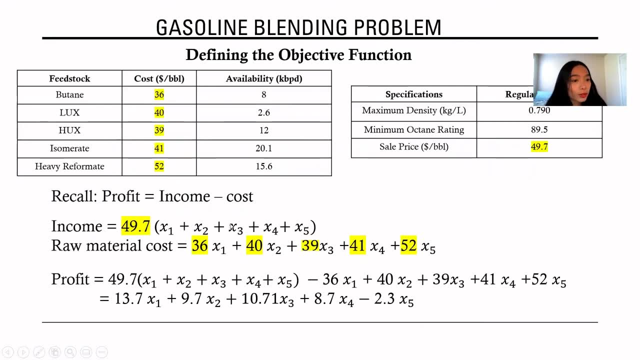 problem, And so our objective in this case is maximizing profit, And therefore we want to make an objective function for profit. So recall that profit is the difference between income and cost, And so let's make a mathematical formulation for income and cost. So income, in this case, is: 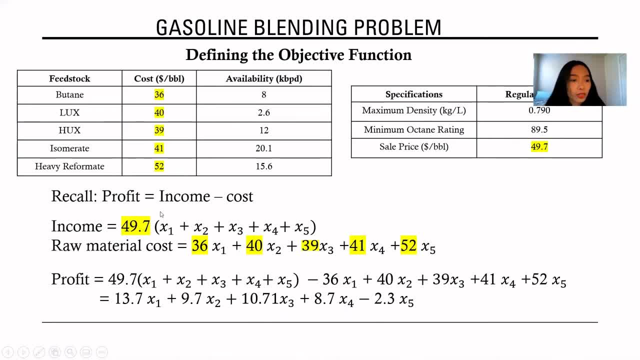 going to be the sale price for the gasoline- $49.7 per barrel, multiplied to the composition of our desired gasoline, which right now is unknown to us. The raw material cost is going to be the product of the cost for each of these feedstocks per barrel times the composition of each of our 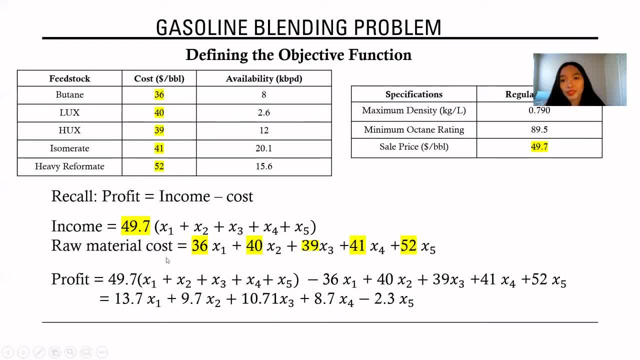 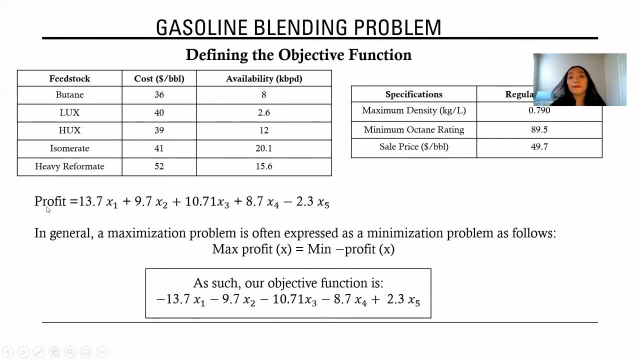 feedstocks, And then we sum that together to get the raw material cost. Taking the difference, we get a mathematical expression for the profit. And so from there, this is our mathematical formulation for the profit, But it is important to note that a maximization problem tends to be: expressed as a cost. So a maximization problem tends to be expressed as a cost, And so- this is important to note- that a maximization problem tends to be expressed as a cost And so from there, this is important to note- that a maximization problem tends to be expressed as a minimization. 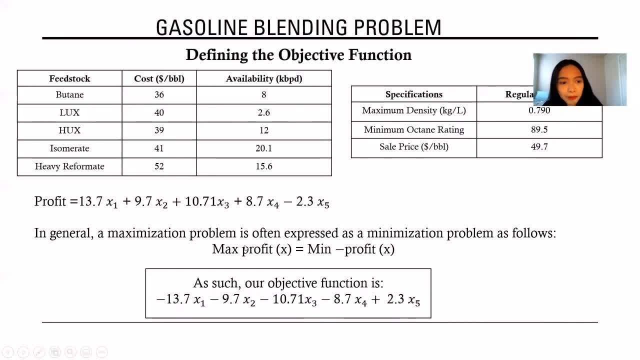 problem, And the way that we do that for this problem is that. so our objective is: you want to maximize profit. Another way of saying that is: you want to minimize the negative profit objective function, And so, since we're treating this problem as a minimization problem, we're going to take the 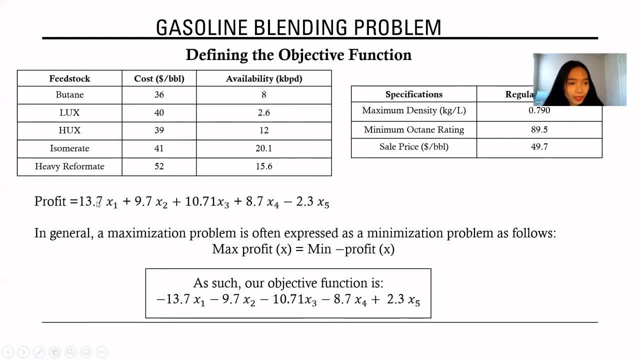 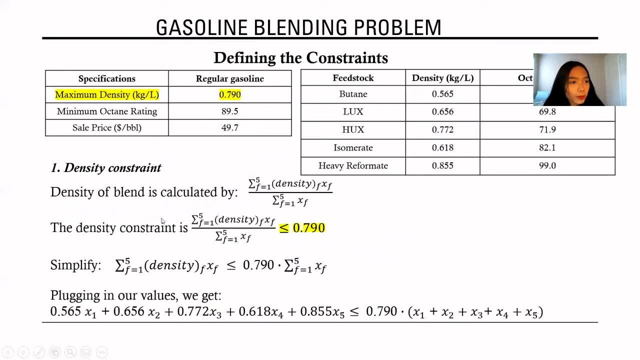 negative of the expression for profit and therefore end up with this expression for our objective function, The density constraint. So we are constrained to have the density of the blend be 0.790 kilograms per liter maximum, And so the way we calculate the density of the blend is through this volumetric fraction expression, wherein the 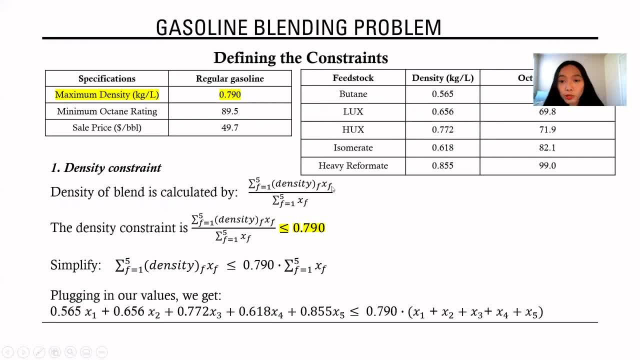 numerator is the summations of the density of each of our feedstocks multiplied by their composition over the summation of all these blend composition. And so, given the density blend, this should be less than or equal to 0.790 kilograms per liter. We cross, multiply and we end up with this expression: 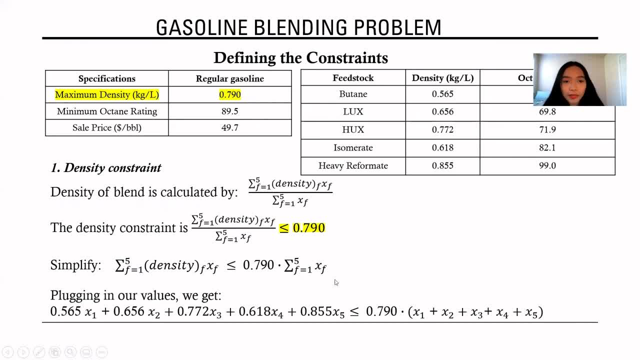 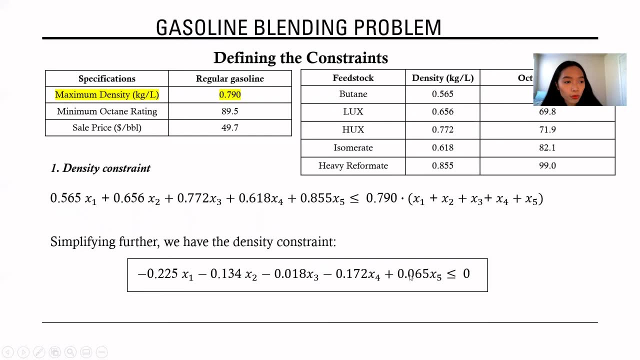 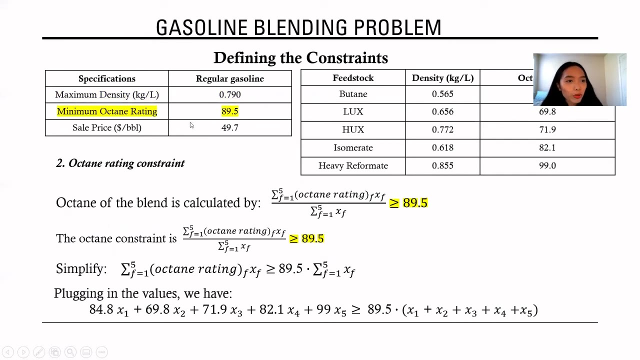 and from here we plug in our values, given information about the density of each of our feedstocks, multiply that to their composition and carry out the rest of the math to eventually get this density constraint. So this is our expression for our mathematical expression for our density constraint. We now move on to the octane rating constraint. So our regular gasoline. 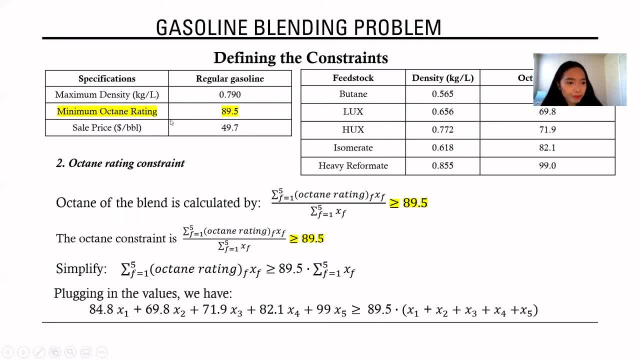 must have a minimum octane rating of 89.5.. And so the octane of the blend is represented by this expression, similar to that of the density of the blend, wherein the summation this time has octane rating multiplied to the composition. 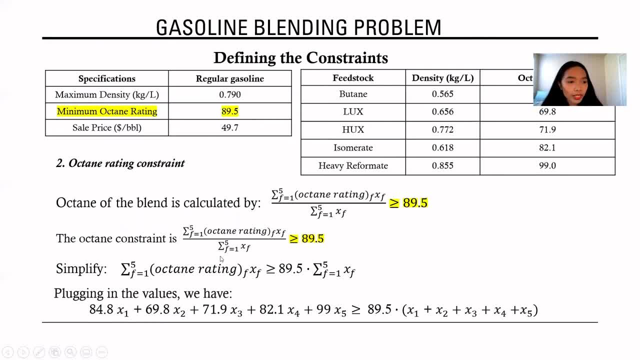 of each of the feedstocks instead of density, And so we know that this octane constraint is the octane of the blend- should be greater than or equal to 89.5.. We do the cross multiplication and end up with this mathematical expression, So knowing what the octane rating is of each of our 5.5. 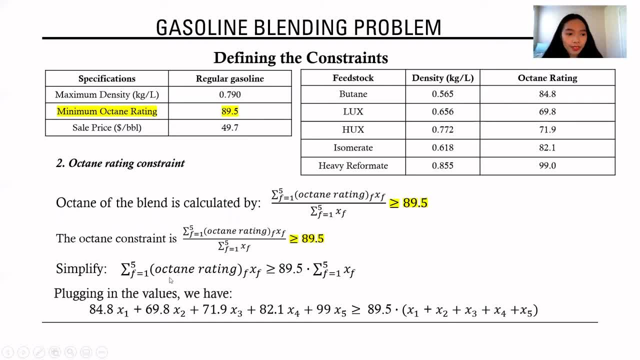 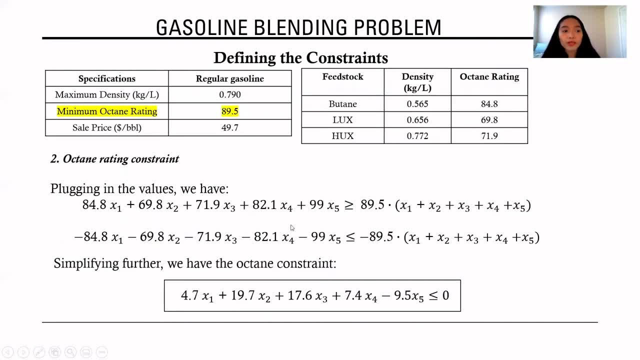 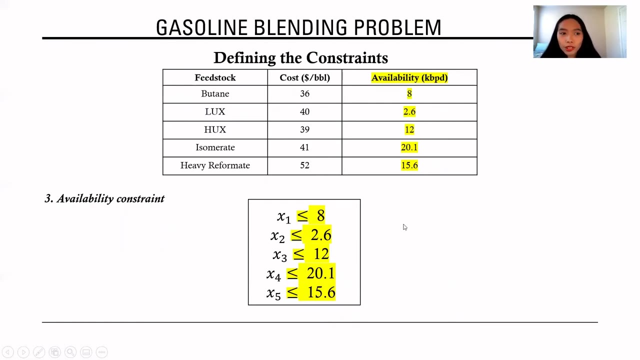 feedstocks and our food stocks. we plug them in as necessary to be able to end up with this expression for our octane constraint And then, simplifying further, we get this mathematical expression for our octane constraint for the gassing blending problem. Our last constraint is the availability constraint, So we are limited to how much of 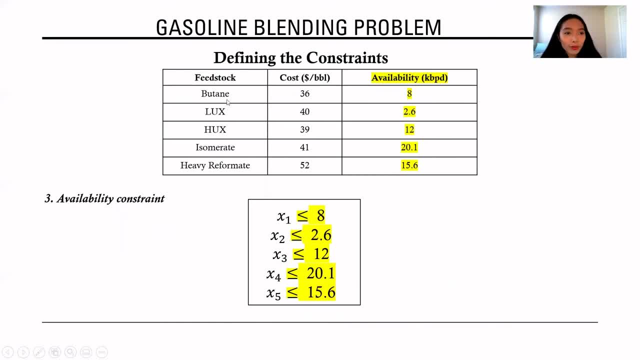 each of these feedstocks we can use, And so in this case, feed 1 is limited to 8.15, equals 6.3 мира per liter, And in that case feed 1 is at least quantified, and in this case feed 1 is quantified. So both of these feedstocks would be 20 Grams per liter. So accordingly we get 60, 30 grams of foodstocks needed in the Yougurt become downloadable variant if onions and other food state- To compare that with the symptoms of digests- are tough for the costing and treating these bindings, of these predictors. 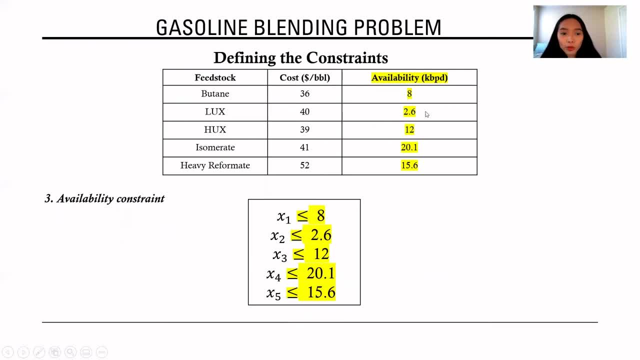 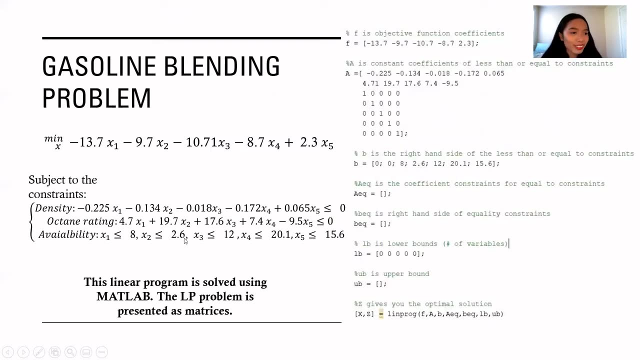 to 8 kilobarrels per day. LUX is limited to 2.6 kilobarrels per day, and so on and so forth, as you can follow along on this mathematical formulations. So the gasoline blending problem, Our overall gasoline blending problem, looks like this: 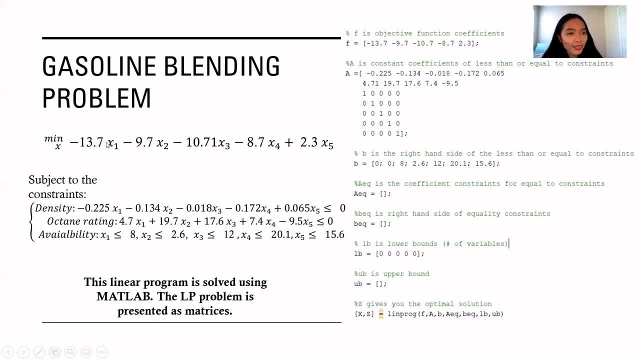 So our objective function is here. Recall that this is the same as negative profit and minimizing the negative profit is the same as maximizing profit. We have our density constraints here, our octane constraints and our availability constraints. So, in summary, we want to find our decision variables X that minimizes our negative profit. 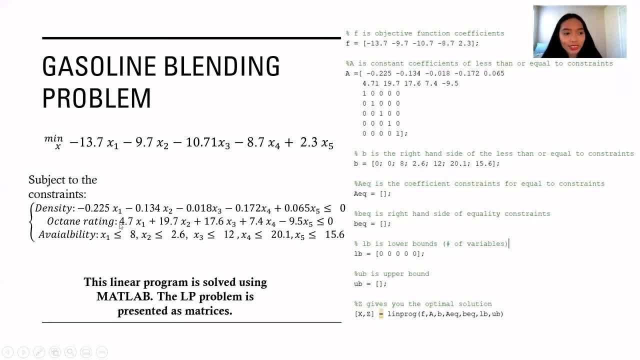 given that it needs to satisfy the density constraints, the octane constraints and the availability constraints to be able to determine the optimal amounts of each of the 5 feet stocks that we need to mix together to acquire the desired gasoline with the desired profit. 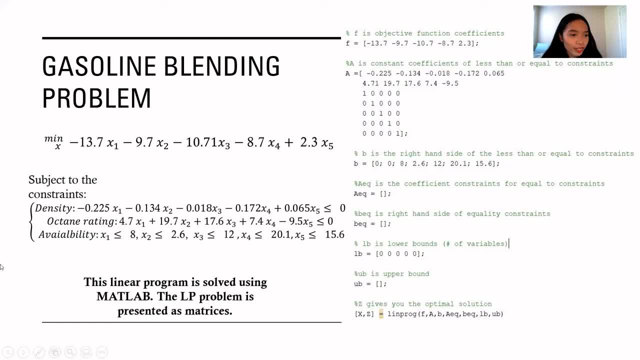 and the maximum profit. So I carry out this linear programming problem using MATLAB. MATLAB has an LP solver that I use to be able to solve this linear programming problem, And so, if you look to the right, I represented each of these expressions as matrices. 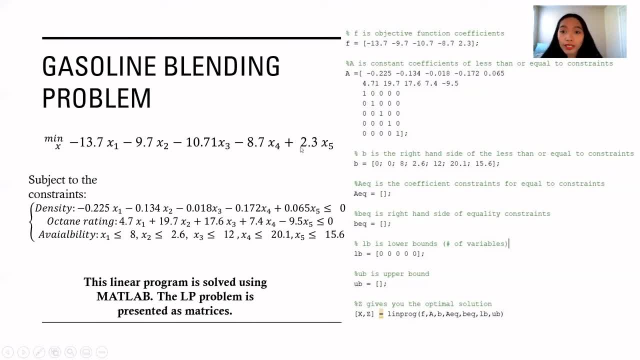 So matrix F contains the coefficients of my objective function. So we have negative 13.7,, 9.7,, 10.71,, 8.7,, 2.3.. We have the matrix A that contains the coefficients of our constraints. 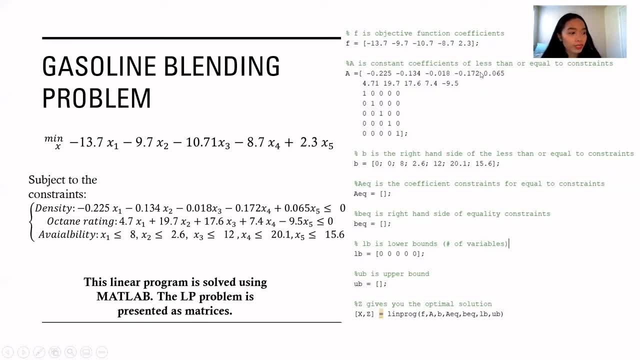 In this case, this row, row 1,, refers to the coefficients of the density constraints. The coefficients of the octane reading are in the second row And this row the third row up until seventh row. these refer to the availability constraints for each of our feet. 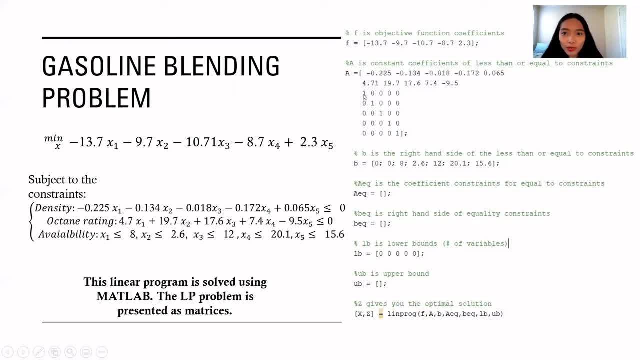 So this is X1, this is only looking at the constraint of X1.. This is only looking at the constraint of X2, X3, X4, X5.. So the matrix B here refers to the right-hand side of the constraints in A. 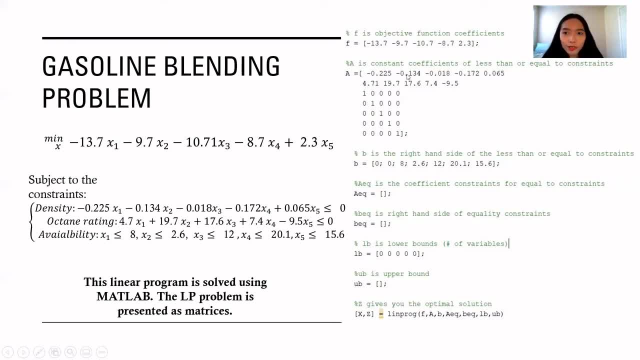 So, as you can see, for the density constraint, which has the coefficients in the first row of A, its right-hand side, 0, is here the first element of B, And then for our second constraint, octane reading coefficients of it being here: 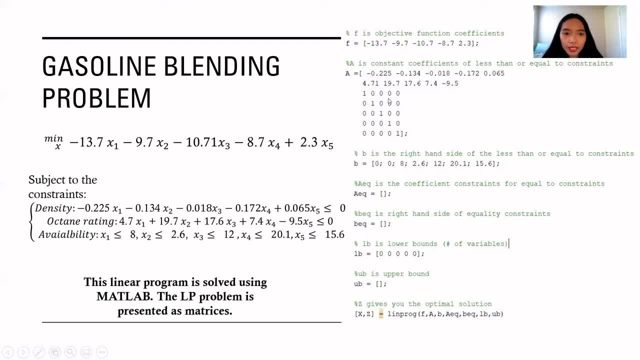 the right-hand side- its right-hand side is here- 0.. And then for the availability constraints, as you can follow along on the right-hand side. for each of these, it follows the order of 8,, 2.6,, 12,, 20.1, and 15.6,. 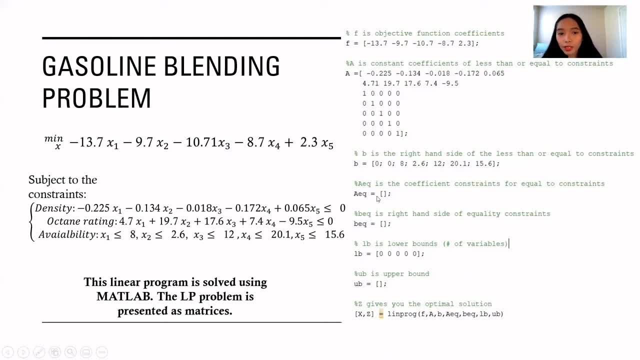 as we can see here, And then we don't have any quality constraints, So we leave AEQ and BEQ blank. The lower bound for our decision variables X is 0 for feeds 1 to 5.. And the upper bound is not limited for our decision variables. 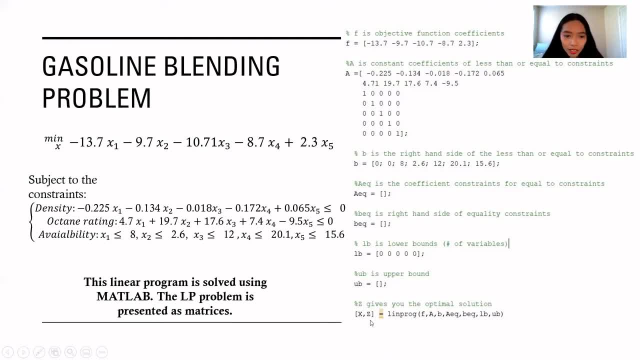 So we leave that matrix blank, And so this is how you call the LP program in MATLAB. So X, in this case, is our decision variables for the five feedstocks. Z, in this case, is going to represent our maximum profit. So calling upon all of these matrices and plugging them in the solver. 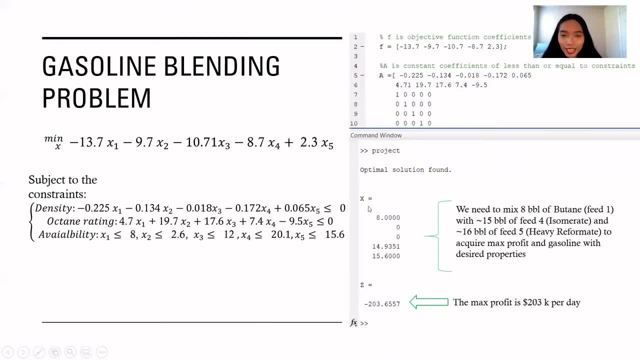 we get this solution, And so this tells us that when we mix eight barrels of butane with 15 barrels approximately, of the isomerate and approximately 16 barrels of heavier formate together, we acquire our gasoline with the desired properties and with a maximum profit obtained of $203,000 per day. 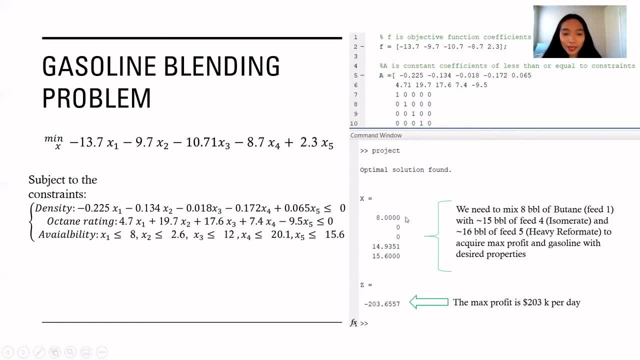 And so this is our optimal blending recipe With the maximum profit that we acquire, And so that's how powerful the MATLAB solver for linear programming can be. It will definitely take much longer if we solve it manually, And so computational techniques such as this really speed up the solutions. 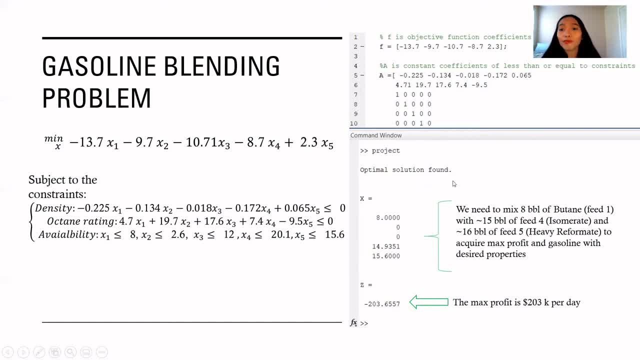 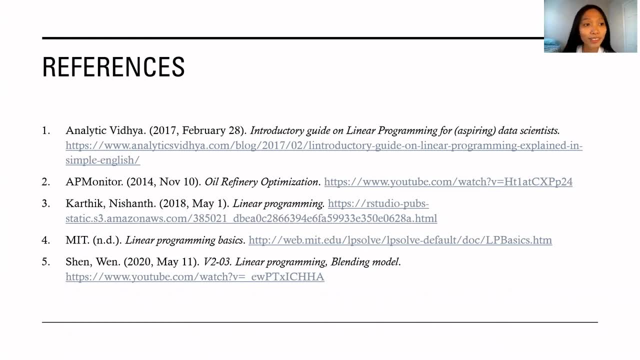 for linear programming problems, such as the gasoline blending problem that we just solved right now. So here are my references that I've used to be able to compile all of this information regarding linear programming, And feel free to look up these sources if you want to learn more. 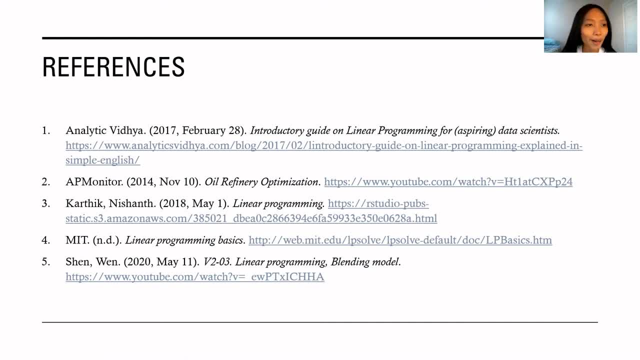 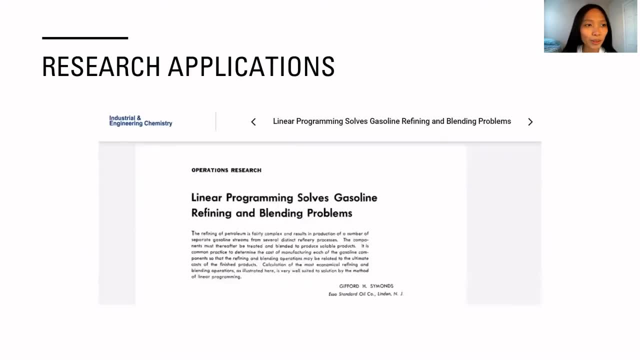 about linear programming and its applications. The last thing I want to cover is the applications of linear programming to different fields. So the first one we're actually going to cover is similar to the refinery blending problem that we've already encountered. So this paper: linear programming solves gas. 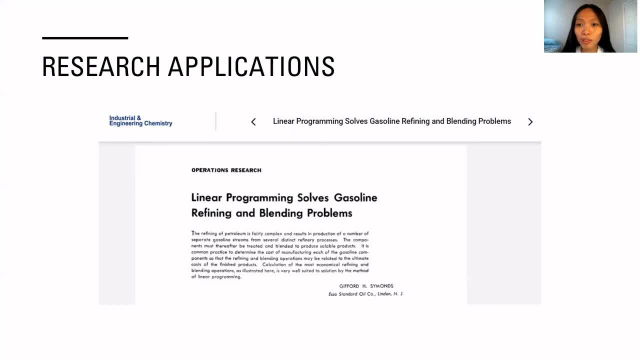 and refining and blending problems, uses linear programming to maximize the profit of the refinery operation, specifically for gasoline production. So that's similar to what we went over in this presentation, But one of the main differences being is that the scale of this optimization problem.